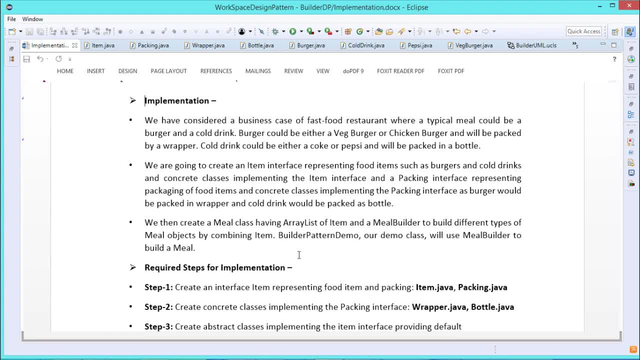 and pattern, and we have considered one business case of fast food restaurant where a typical meal could be a burger and a cold drink. a burger can be of two types, that is, a veg burger and chicken burger, and which will be packed by a wrapper. and cold drink could be either, say, coke or pepsi, and 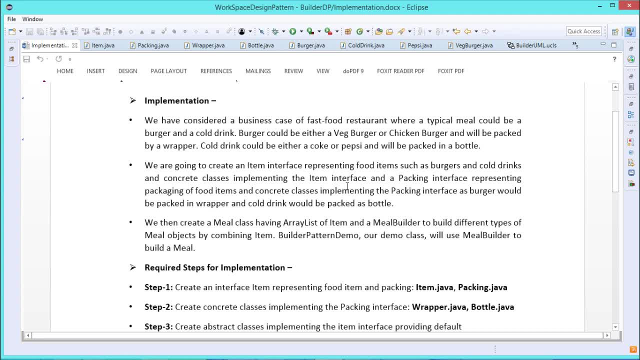 will be packed in a bottle. so here we are having two items in in our meal. one is the burger, another one is the cold drink. burger can be of two types: veg burger and chicken burger, which will be packed in a wrapper. and cold drink can be of two types. one is the coke, another one is the pepsi and will 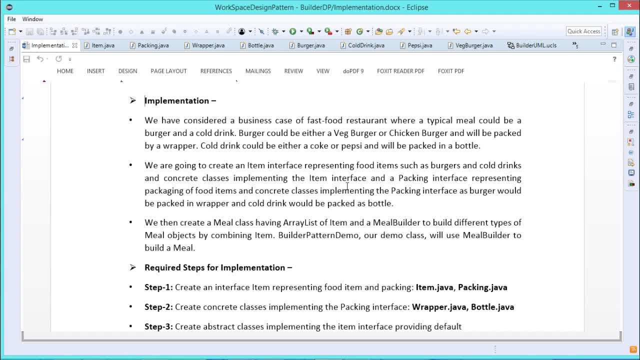 be packed in a bottle. so we are going to create an item interface representing food items, such as the burgers and the cold drinks, and concrete classes implementing the item interface, and a packing interface representing packing of food items and concrete classes implementing the packing of food items and concrete classes implementing the packing of food items. and. 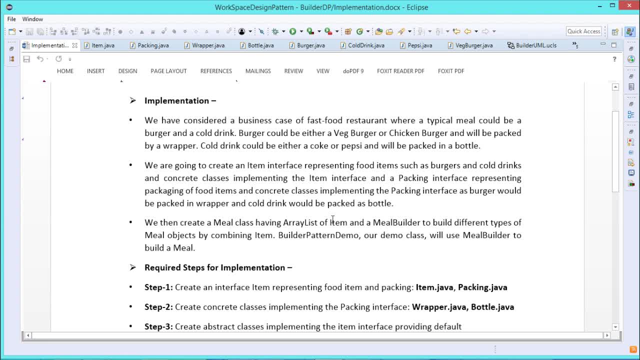 interface, as burger would be packed in a wrapper and, as i told you earlier, the cold drink would be packed, as in a bottle. so we will be having one class, that is, a mill class, which will be having the array list of items and menu and the mill builder to build different types of mill objects. 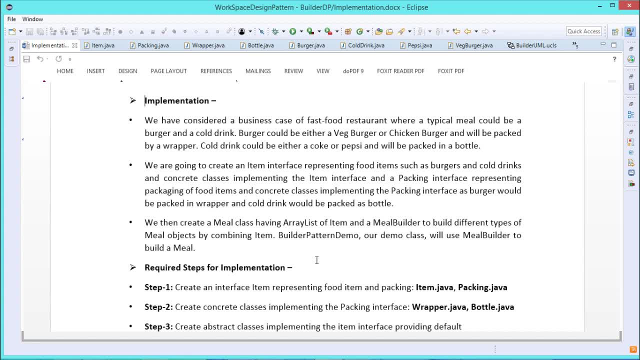 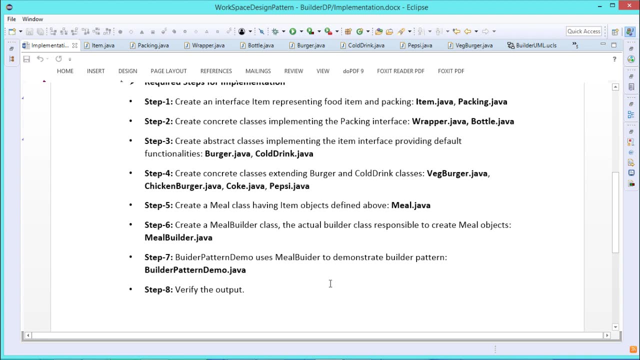 by combining items and builder pattern demo, which will be our demo class and which will use a mill builder to build a mill. so there is a total concept here. we shall be going for the implementation step by step. so step one is that we should be creating an interface item and represent 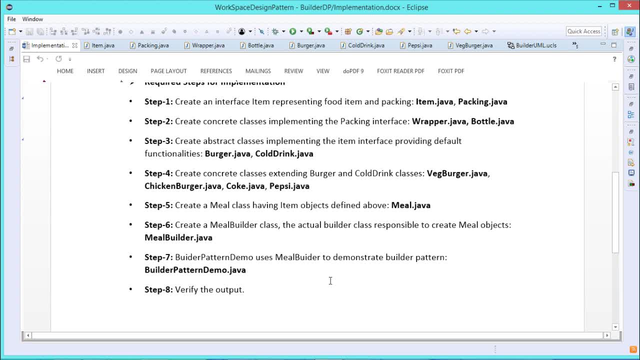 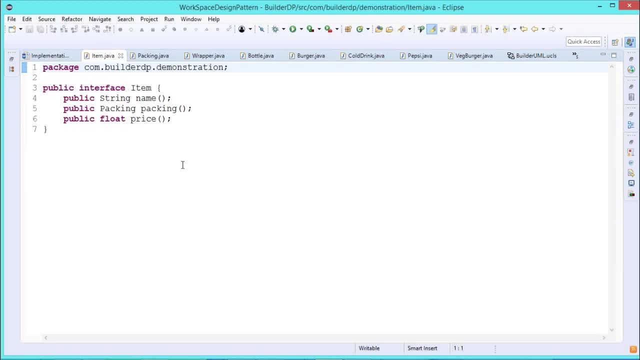 representing the food items and the packing. that is the itemjava and packingjava. so let us go for the item at first. so this is our item. you can find that. so public interface, item. so item is nothing but one interface having got this public string name. so name is one method, returns a string. packing is another method which returns a packing. 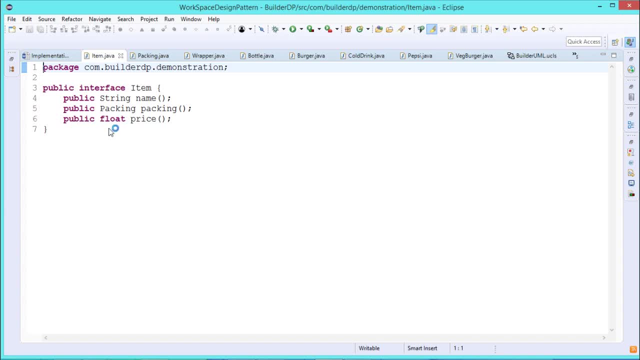 and here we are having. the price is another method which returns applied price in the terms of or of the type of float here. so here we are having one interface, known as the item, which we which is having three methods are: their name, which returns a string packing, which returns a packing class. 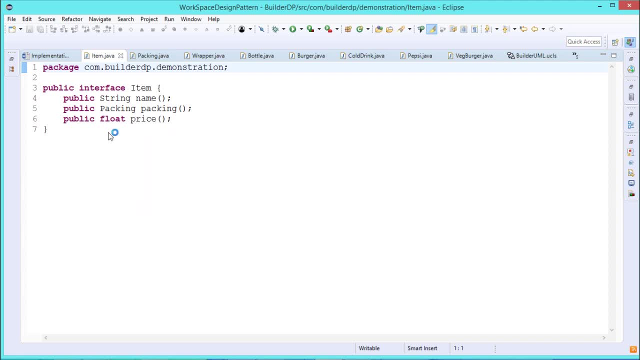 object and we will be having the price, which will be returning a float data. so here you see, we are having this packing as one interface here. this is item- is actually returning this packing, this particular interface object rather, and this method is packing and this interface has been defined here. so this particular interface packing is having one method, that. 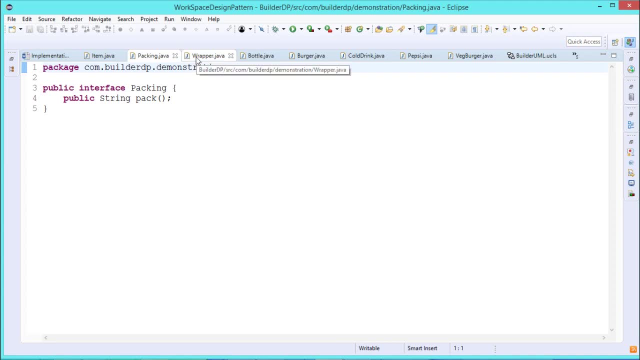 is the pack which returns a string here. so that is where having this thus rapper, this rapper is implementing this packing. so packing is one. packing is one interface which is having only one method defined. that is our pack. so wrapper is going to write the body for this. 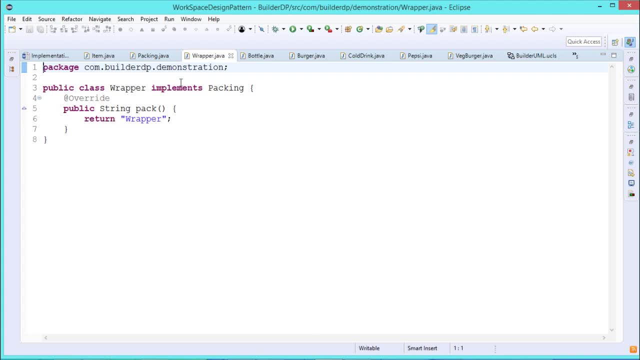 method that is a return wrapper. so this is a wrapper which is implementing this packing interface. bottle is another class which will be implementing this packing interface and here the respective pack method is returning the string that is the bottle. so this is our item interface. we have discussed that one. this is our packing interface. we have discussed that one and this. 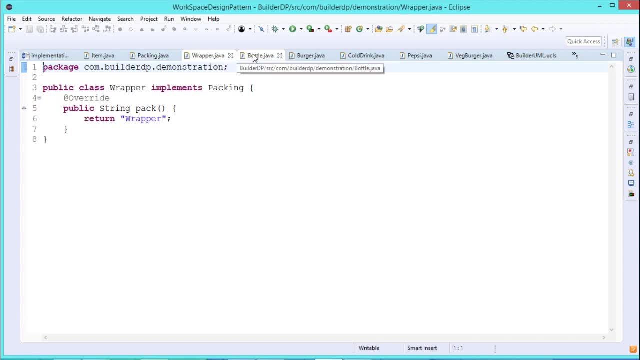 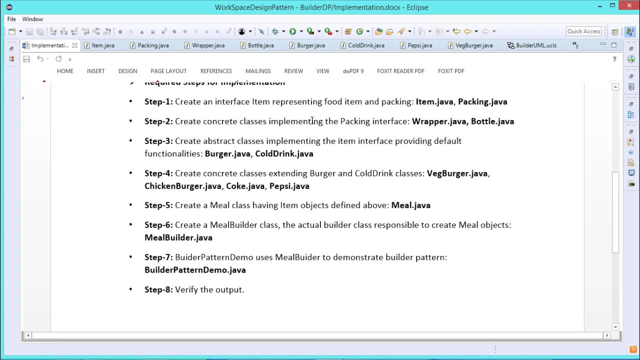 is a wrapper class implementing packing interface. bottle class, which is implementing the packing interface. okay, now create concrete classes implementing the packing interface. that is a wrapperjava and bottlejava. so this up to this part, we have done so. create abstract classes implementing the item interface providing default functionalities: that is a burgerjava. 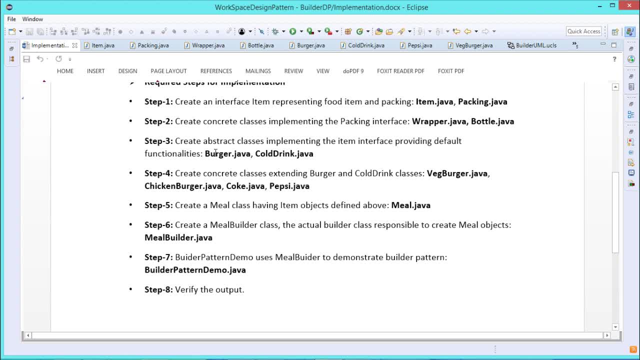 and cold drinkjava. so item can be of two types, that is, a burgerjava and cold drinkjava. and we know that this particular create concrete classes extending burger and the cold drink classes. and we know that burger will be of two types, that is, a veg, burgerjava and chicken. 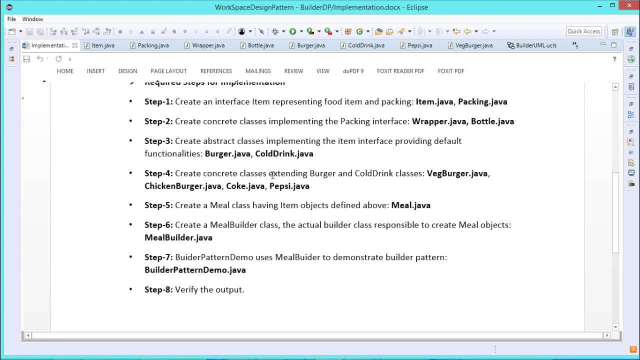 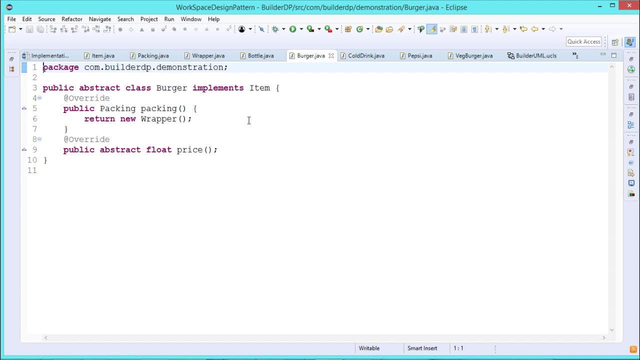 burgerjava, representing veg burger and chicken burger here, and cold drink. this particular is having two types: one is a coke and the pepsi, so respective classes will be cokejava and pepsijava, so let us go for that. so here we are, having this burger, so which is implementing? 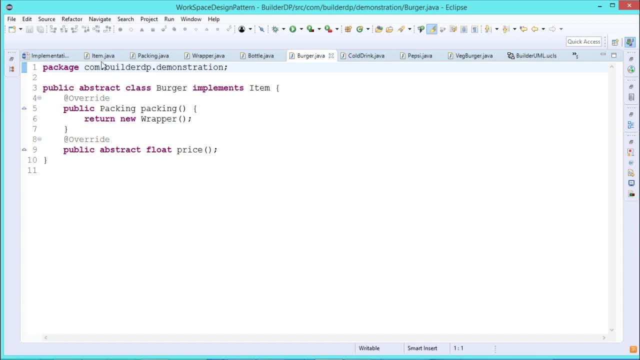 this item. this burger is implementing this item. we know that, in case of item, we are having this name method, we are having this packing method, we are having this price method. so, in case of burger, we are just writing this packing here. so this is a abstract class burger. 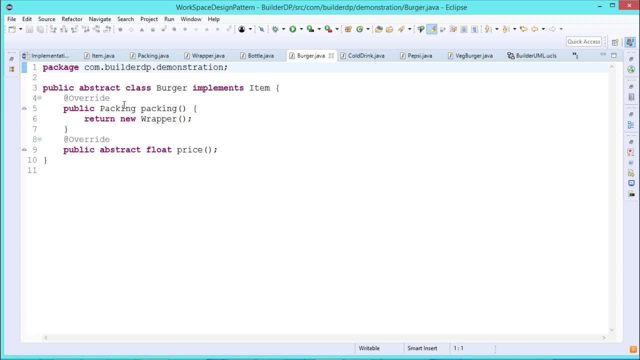 implements item so as it is abstract class. so here we are overwriting the method. there is a packing returns new wrapper, returns new wrapper and we are having this public abstract float price here. so this item, we are having this price, we are having this float, we are having this. 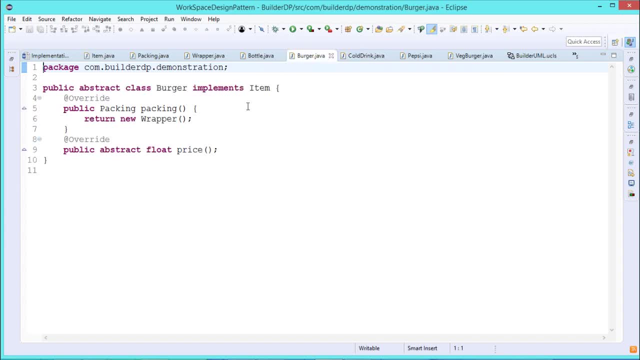 packing, we are having this name and here we are having this burger. here we have defined that one accordingly, which is so burger is nothing but one abstract class which is implementing item. next, we are going for this cold drink, so cold drinks is also another abstract class which is implementing. 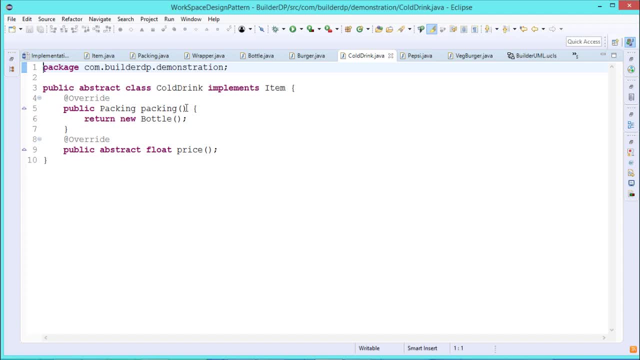 the interface item and here this particular method, packing. we have written the body for that: return new bottle. so in case of burger returns new wrapper, in case of cold drink it returns new bottle. so now we will be going for this pepsi, so these are pepsi here, so which extends the cold. 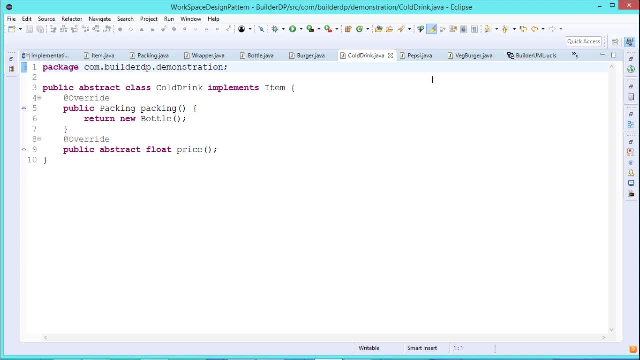 drink, so this is a cold drinkjava. we know that this is the abstract class, so this is a pepsi which is extending this cold drink here. this price, we are over. adding this price method, the return value is 35.0 in the. in the. in the. 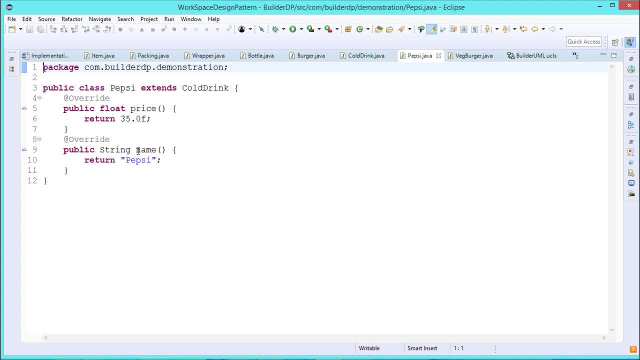 the data type of float in the type of float and there is a name method, is also getting overwritten, so it returns a pepsi. so in case of pepsi, we are having this. so now let us go for our coke here. so we are writing this coke mentioning the price, and the coke returned as a, as a string here. now we 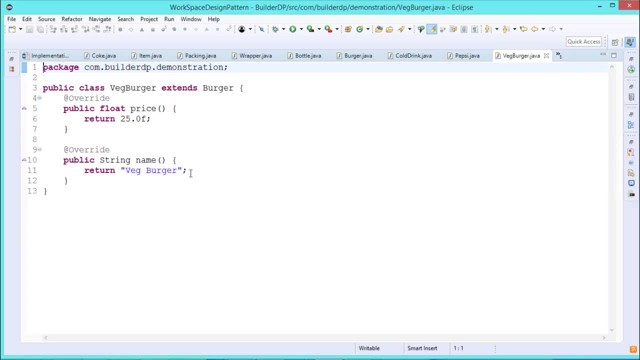 shall go for this veg burger. we can go for this veg burger which extends burger. so you know that burger is nothing but one abstract class here. so that is a abstract class. burger implements items. so we are going for this veg burger and here we are just defining this method, the price which 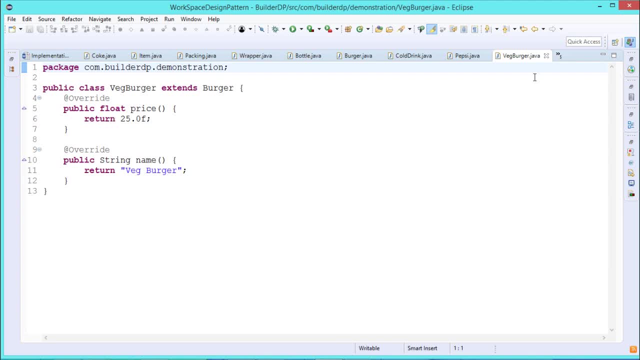 returns this value and name as the veg burger. so now let us go for the chicken burger here. so this is the chicken burger, which extends the burger mentioning the price and the respective name which will be returned in the as a type of string from this method name here. so now, 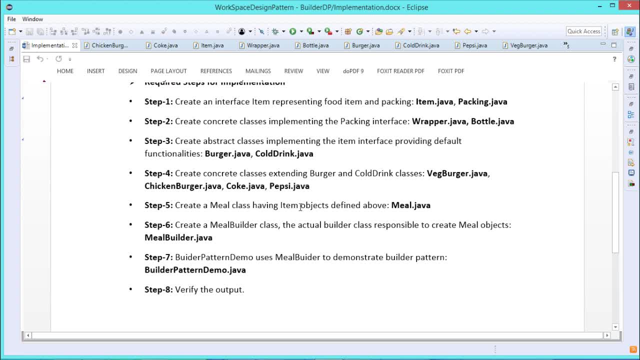 understand the affection. so now let us go for the chicken burger, which extends the打差 to to this part. we have done so. now create a mill class having item objects defined. above there is a milljava, and then we'll be going to define one mill builder, so this particular mill builder. 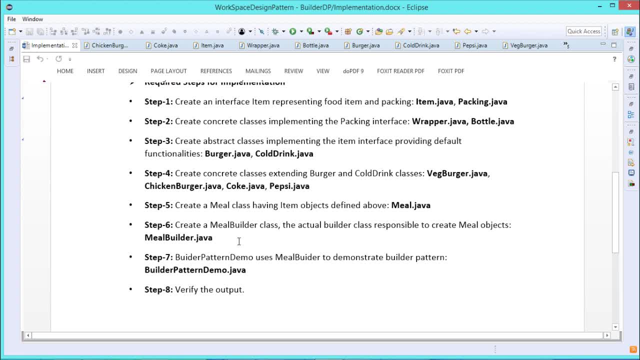 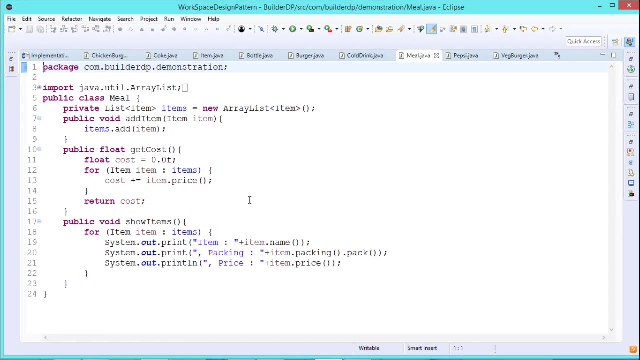 class. that is the actual builder class responsible to create the mill objects, and we will be having the last class. there is a builder pattern demo which uses the mill builder to demonstrate the builder pattern here. so now we will be going for the mill. this is our milljava. so here we have used one arraylist of items. there is a new arraylist item. 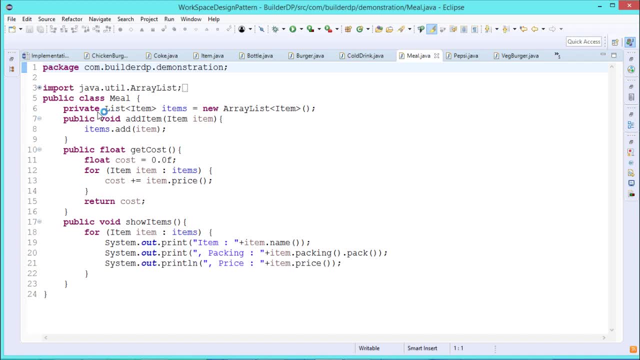 it will be holding the item objects in this arraylist and we are having this add item, which will add items to this arraylist items, and we're having this get cost. so initially i'm just initializing cost with the value of zero float and then for each and every item, whatever we'll- 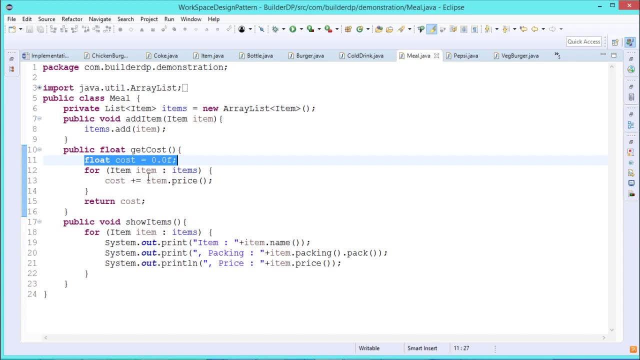 be having in this, in this arraylist, the respective prices are going to be added and the final cost will be returned of the type float. we're having the shore items, so using this, for each so item, object, item which will be found in this items at a list, the respective name, the packing dot pack, and then we are having this. 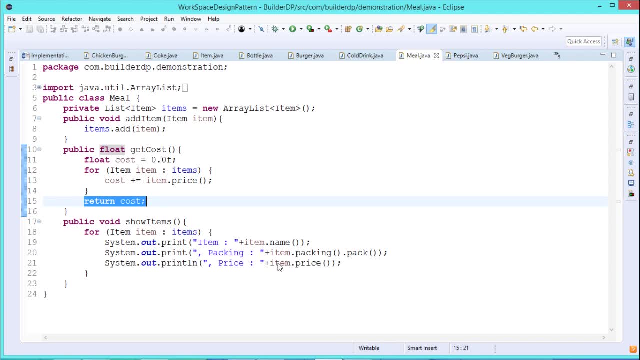 price. so item dot packing method, dot pack method and this item dot price method, which will print the respective price packing and the item here. okay, now we'll be going for the next one, the next one, the next item going to be called for, the next item, the next item here, this is going to be: 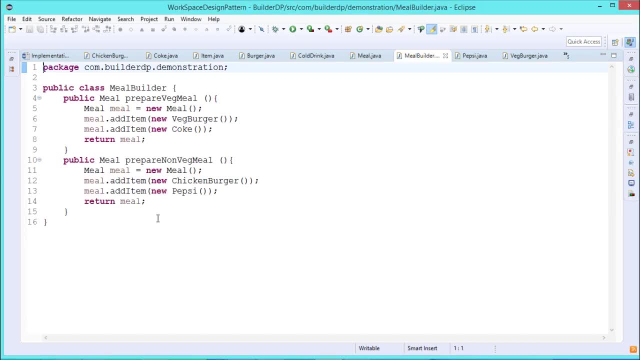 is the menu builder. dot. java, this is our menu builder. it is having two methods. one is the prepared veg meal and prepared non-veg meal, so meal. so this is a meal we are having, so its object has been defined here. meal meal is equal to new meal, so meal dot. add item: new veg burger and meal. 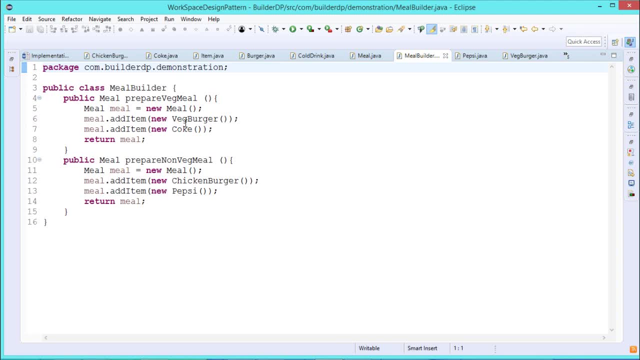 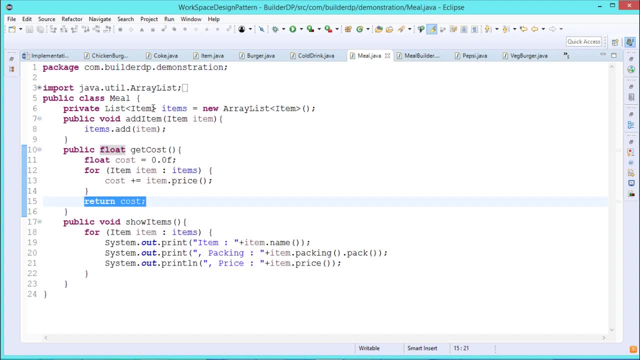 dot add item new cook. so respective objects, which will be respective objects, will be added with this meal. so you know that this meal is having actually one add a list, that is the items. so there these objects are actually going to get added, because you know that in case of item add, 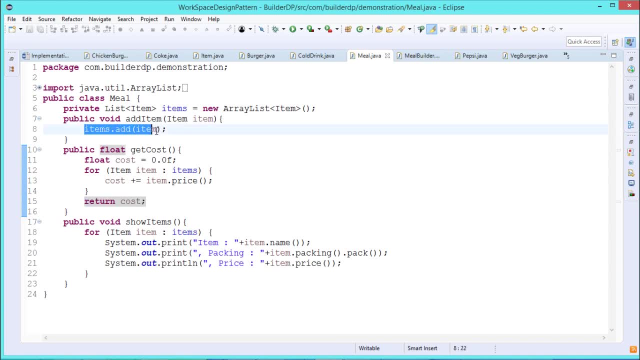 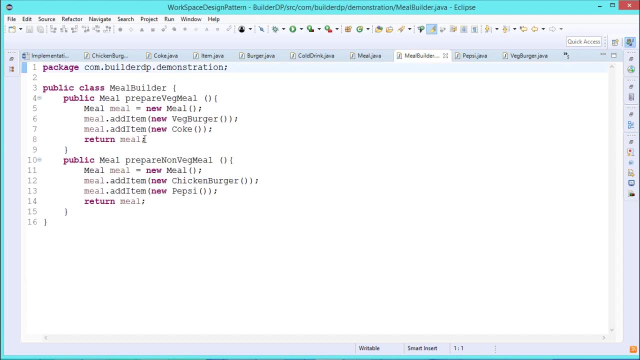 item. in case of add item, this items dot. add item. we have written. so whatever the parameter we are passing here, objects we are passing here, they are going to get added into that add a list defined under this meal class. so return meal in case of prepared non-veg meal will be taking this. 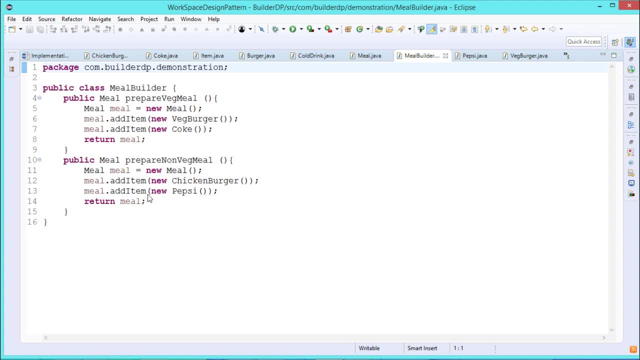 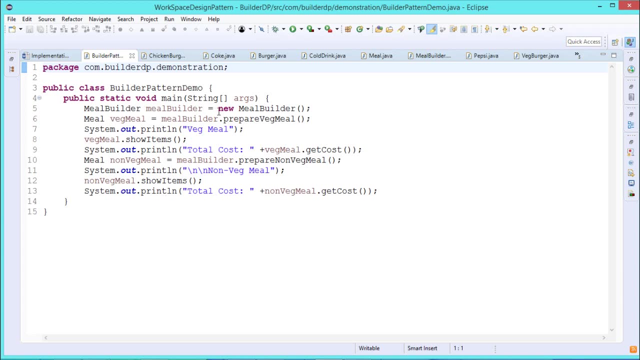 these chicken burger here and we are going to add this pepsi object there. so the last one, that is our demo builder pattern demo. so which is which is defining one menu builder is equal to new menu builder. so we are defining one menu builder class object here and then we are going for the prepared 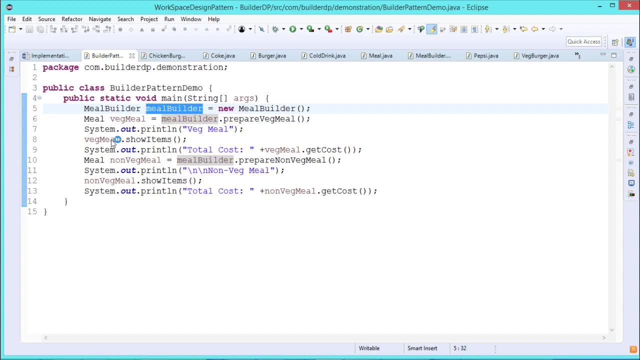 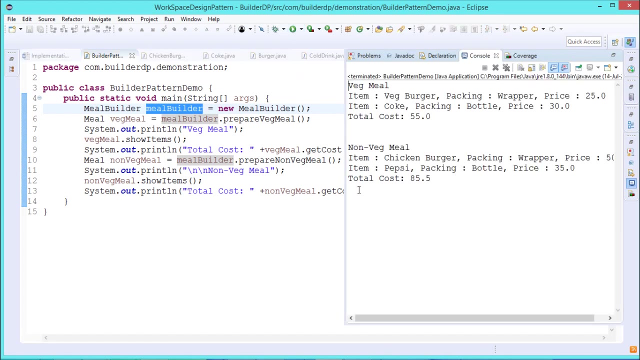 veg meal. so systemoutprintln veg meal and then veg mealshow items. it will print all the items which will be included in the veg meal and then for the non-veg meal, the items are to be printed and the respective costs will be also getting printed here. so now let me execute my 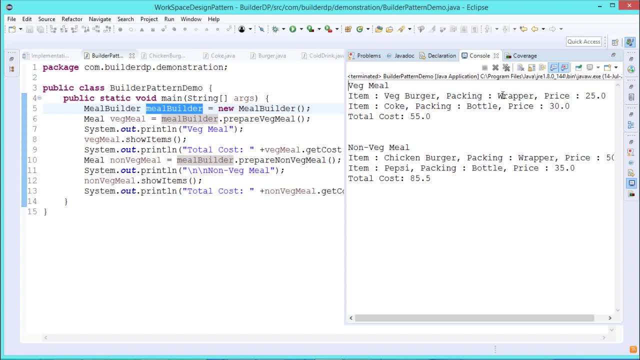 code. so in case of veg meal, item is veg, burger, packing is equal to wrapper, price is equal to this, item is equal to coke, packing is bottle and the price will be this and total will be 25 plus 30. there is a 55 here and for the non-veg meal also, we are having the chicken burger packing. 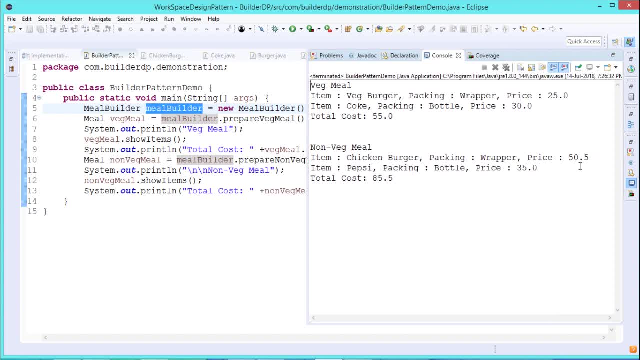 wrapper price is equal to this and total will be 25 plus 30. there is a 55 here and for the non-veg meal is equal to. we can also get the price. the price is 50.5 and item is pepsi packing bottle and price. 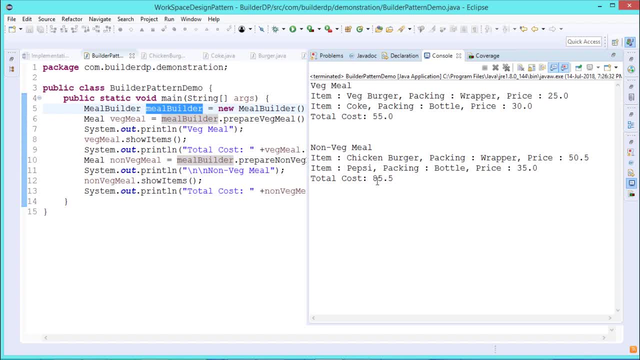 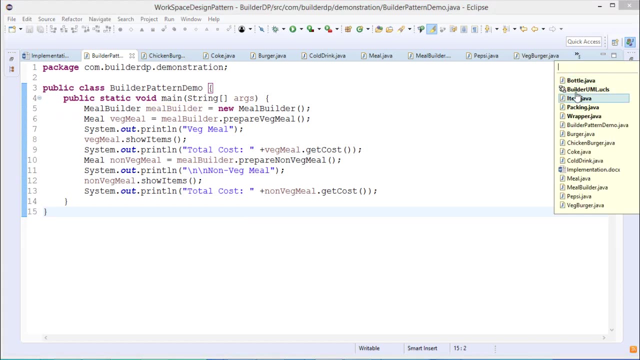 is 35, 35.0, so if you go on adding, it is 85.5 here. so in this way, in this particular demonstration, we are just showing that: how to define different classes for the implementation of this builder design pattern. so now let us go for. now let us go for the. this is a class diagram we are getting. 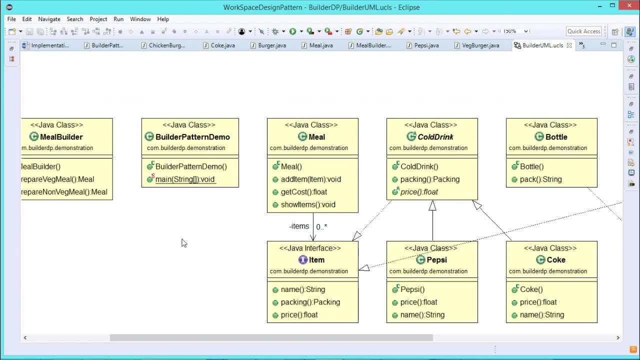 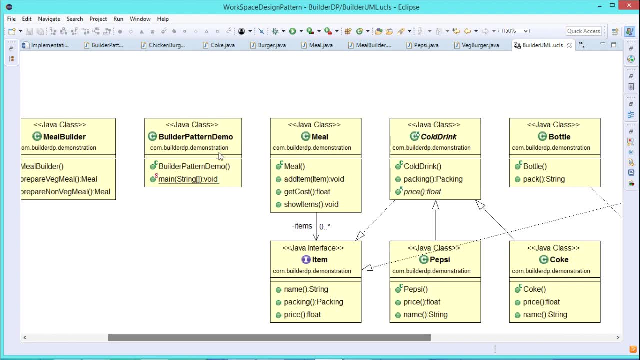 here. this is a class diagram, so this is the mill builder you are getting here. there is a java class builder pattern demo. this is the constructor we are having. this is the main function under the public scope of type static. this is about mill. you can find that this is a mill. 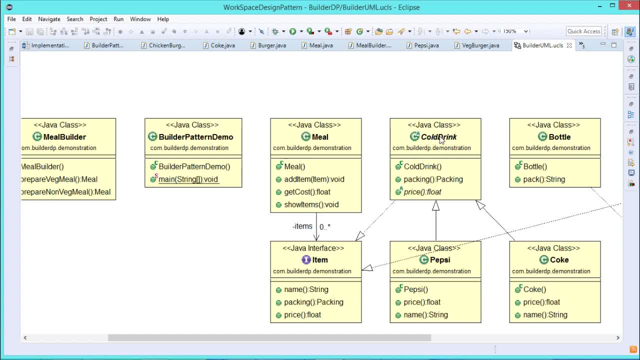 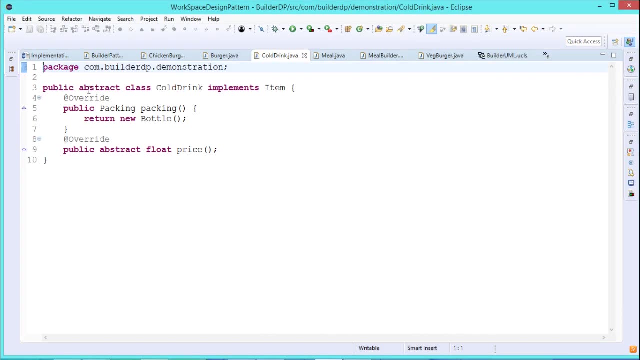 add item. there is a get cost and show items. we are having. there is a cold drink. this cold drink is nothing but one java class here and we are having this pepsi and the coke you can. you can easily find that this cold drink. you can just let me go for that. there's a colding, is there? so colding is of the type abstract class.